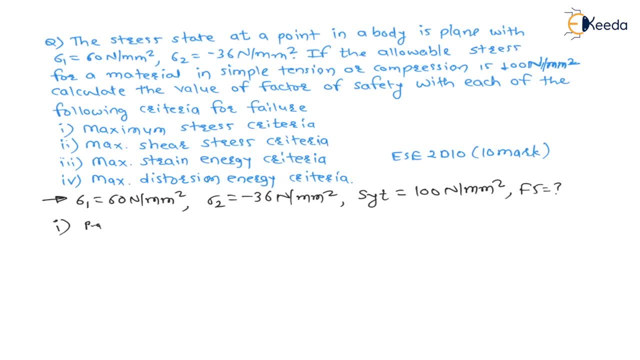 First of all, maximum stress criteria. maximum stress criteria means Rankine theory. Maximum stress criteria is nothing but Rankine theory, normal stress, which is nothing but. here. sigma 1 is used for the design and, as per this theory, sigma 1 is equal to right. maximum normal stress is equal to s y t divided by factor of safety. 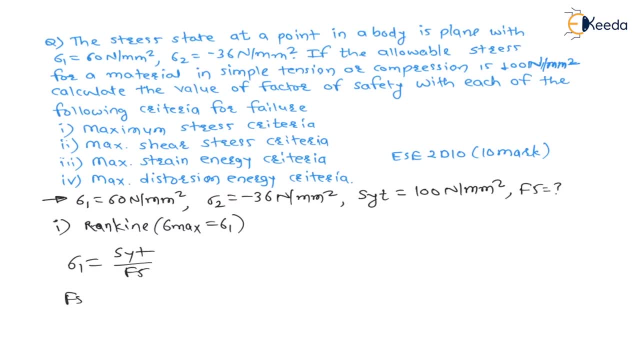 s y t divided by factor of safety. therefore, factor of safety is equal to s y t divided by sigma 1. sigma 1, which is nothing but 100, divided by sigma 1, is given 60, sigma 1 is given 60, and this value 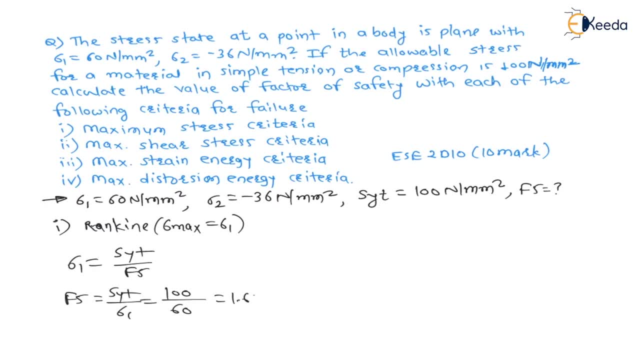 this value you will find as 1.67, 1.67. therefore, factor of safety as per maximum stress criteria is 1.67 right now. second, second criteria is. second criteria is maximum shear stress criteria. that is, this theory is called guest theory or tresca theory. this theory is called guest theory. 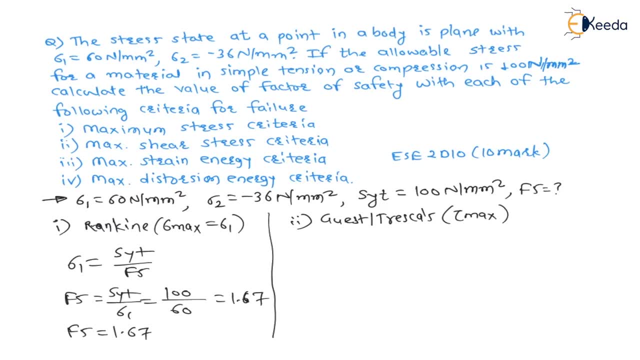 or tresca theory. in this theory, maximum shear stress is used for the design. in this theory, maximum shear stress is used for the design. now this maximum shear stress. maximum shear stress is maximum of maximum of mod of sigma 1 minus sigma 2 by 2. 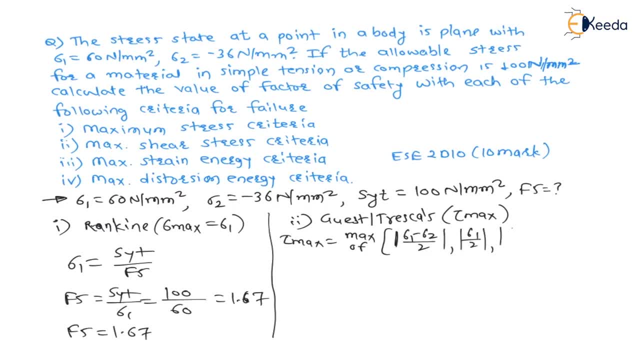 comma, sigma 1 by 2 comma, sigma 2 by 2. now, any one maximum value out of these three values, the maximum value we have to consider. and as sigma 1 and sigma 2 are unlike in nature, that means sigma 1 is tensile and sigma 2 is compressive, means one is positive, other is negative, therefore maximum. 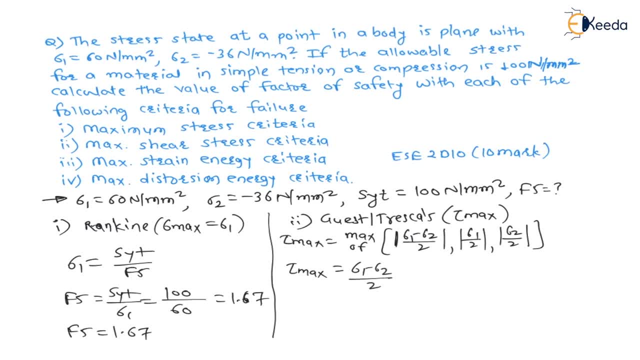 shear stress will be sigma 1 minus sigma 2 by 2, for provided case, therefore, is equal to 60 minus minus becomes plus plus 36 divided by 2, which is nothing. but if you calculate maximum shear stress you will find the value is 48 newton per mm square newton per mm square right and the theory says: 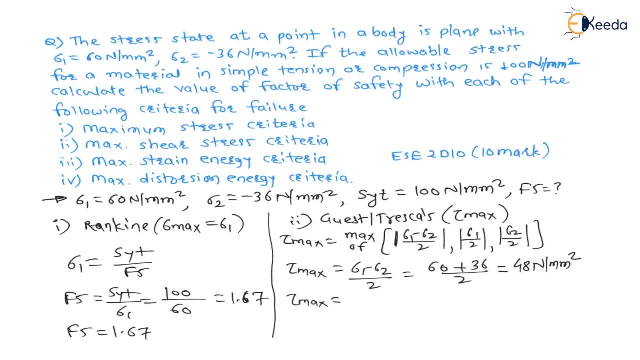 that the theory says that this maximum shear stress is equal to ssy divided by factor of safety, which is nothing but syt divided by two factor of safety. syt divided by two factor of safety, now put the values, put the values. term x is 48 is equal to syt. is syt is given 100. 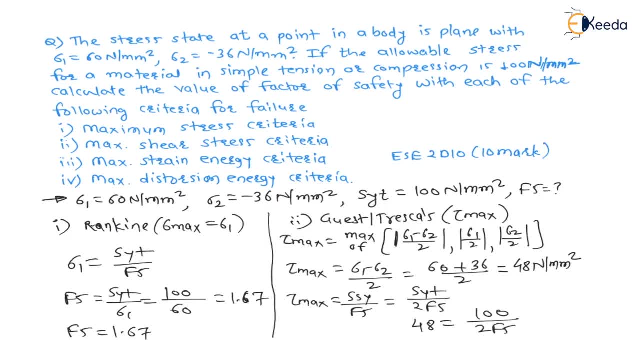 divided by 2 into factor of safety. now if you solve for factor of safety, if you solve this for factor of safety, you will find that factor of safety- for as per this theory- is 1.04. factor of safety, as per this theory, you will get 1.04. right, this is the value as per second criteria. 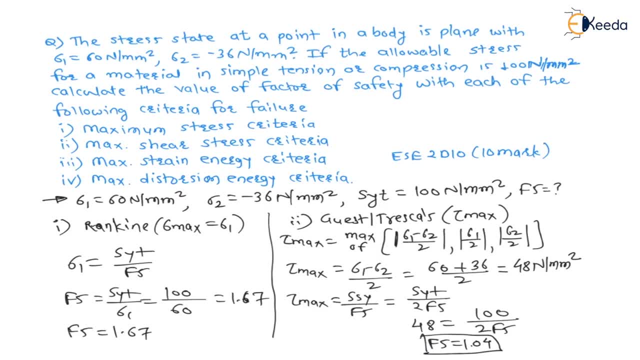 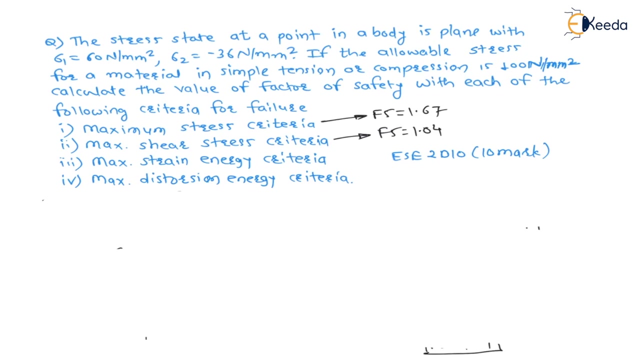 that is maximum stress criteria. therefore, here i am writing, as per first criteria: factor of safety is 1.67. as per second criteria: maximum shear stress criteria- factor of safety is 1.04. now we will solve for next criteria, that is, as per second criteria. as per third criteria: strain- maximum strain energy criteria: maximum strain energy. 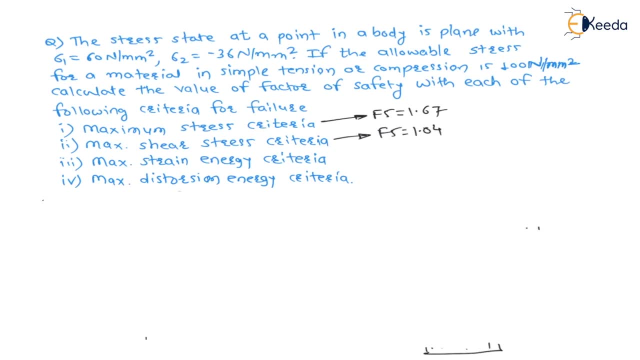 criteria right now: see for maximum strain energy, for max. third maximum strain energy, that is u total Total strain energy. this is a total strain energy. criteria means this is a Higgs theory. this is a Higgs theory. this theory is Higgs theory and, as per this theory, S y t divided by factor of safety is equal to under root of, is equal to under root of sigma 1 square: sigma 1 square plus sigma 2 square minus 2 mu: sigma 1, sigma 2.. 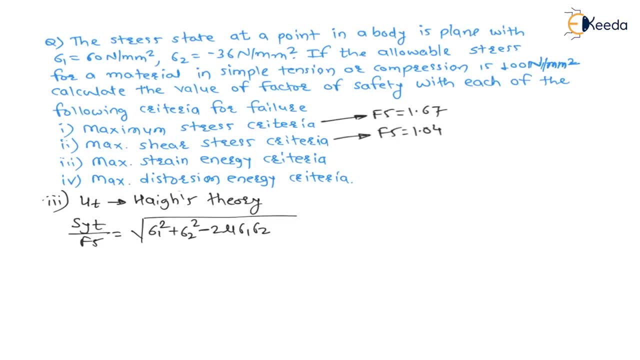 Now, as Poisson's ratio, mu value is not given, therefore assume mu is equal to 0.3, considering steel. as for steel, we are assuming that material is steel and for steel Poisson's ratio is 0.3. this we have to assume here. therefore, put the values S y, t is 100 divided by factor of safety is equal to under root of sigma 1. sigma 1 value is 60 square plus sigma 2 is minus 36 whole square minus 2 into 0.3.. 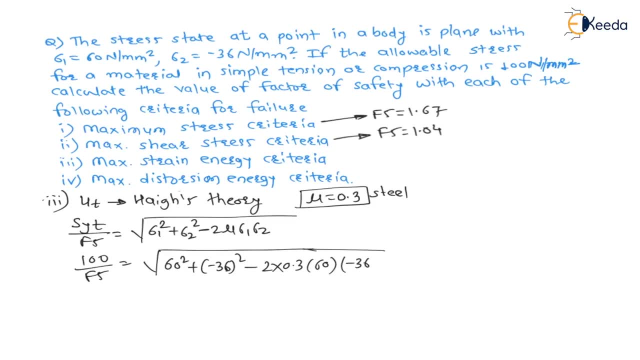 S y t into 60, into minus 36, right and here, if you solve for factor of safety, if you solve for factor of safety, you will find that factor of safety is equal to 1.27. here only factor of safety is unknown. solve for this, you will find that 1.27. this factor of safety you will get. therefore, as per maximum strain energy criteria, you will get factor of safety is equal to 1.27. now we will solve as per last criteria, that is, maximum distortion energy criteria.